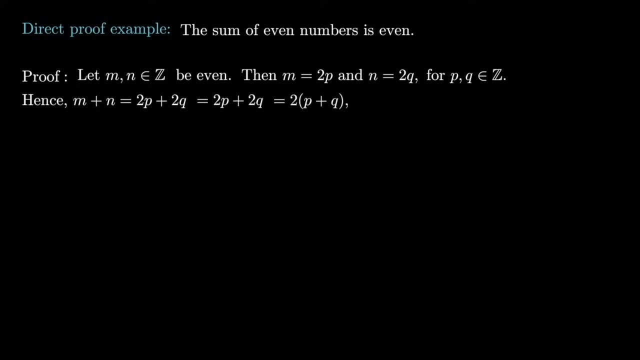 but that's going to be 2 times p plus q, which is a multiple of 2.. Therefore, even Use your knowledge of the previous example to give the following a try. Try to prove that the sum of two odd numbers is even. Let's look at this practice problem. The sum of two odd numbers is even, Assume that m and n are. 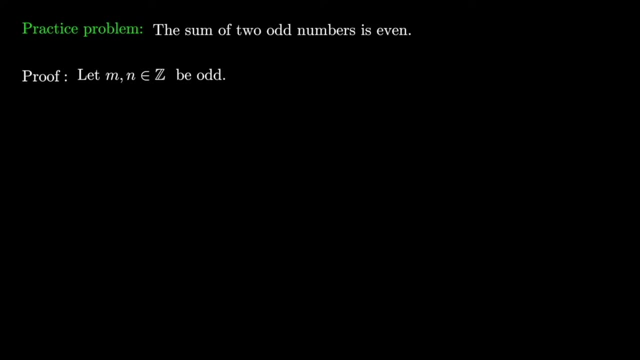 odd. By definition of being odd, that means they're an even number plus one. so we can write m as 2p plus 1 and n as 2q. Now if we add them together, what we see is that m plus n is 2p plus 1 plus 2q plus 1.. 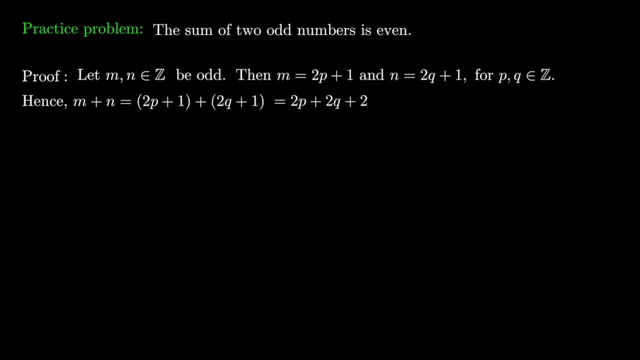 If we simplify this expression, we get 2p plus 2q plus 2.. All of these have a 2 in them, so we can factor the 2 out and write this as 2 times p plus q plus 1.. Now we've shown that m plus n is a. 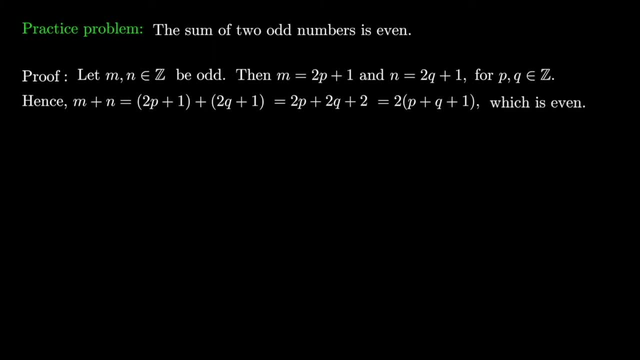 multiple of 2.. By definition, that's what an even number is, And that's it. We'll do one more practice problem just to make sure we really get a grip on these. direct proofs, Again using the same technique, show that the sum of an odd number and an even number is odd. 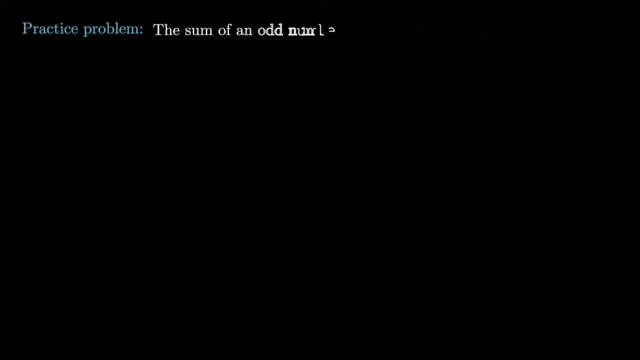 Let's have a look at the solution to this practice problem now. So recall that we need to show that the sum of an odd number and an even number is odd. Proceeding in the way that we usually do, we'll take m and n to be integers. We'll assume that m is even and n is odd. If m is even, then 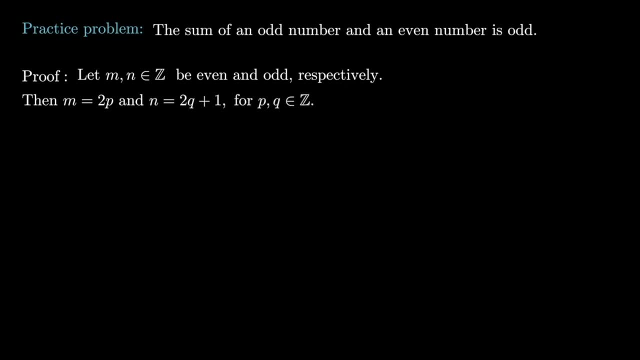 we can write m as 2p for some integer p, and if n is odd, we can write n as 2q plus 1 for some integer q. If we add them up, we see that m plus n is 2p plus 2q plus 1, but that must be 2p plus 2q. 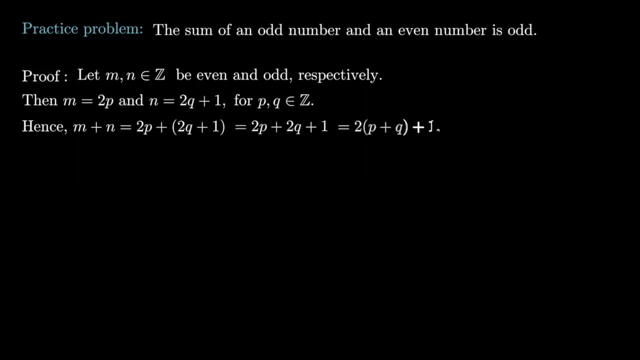 plus 1.. Now 2p plus 2q: both of those have a factor of 2, so that means that 2p plus 2q is even The 1 doesn't have a factor of 2, so we now have an even plus 1, which is odd. you.